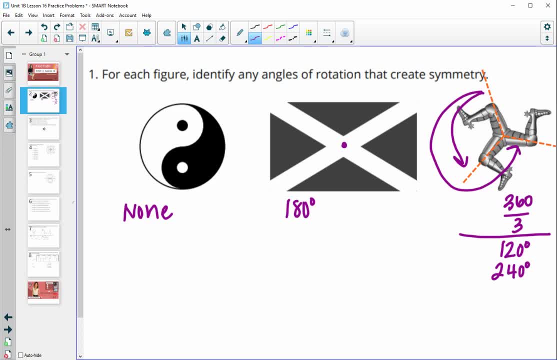 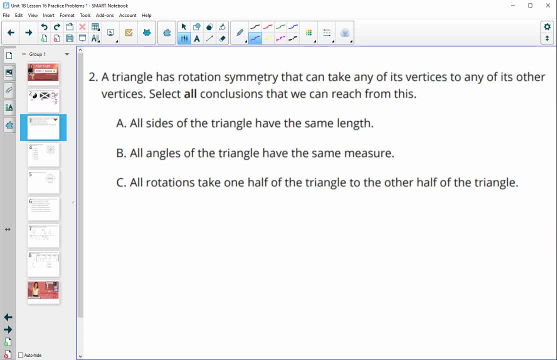 not count as a rotational symmetry angle. number two: a triangle has rotation symmetry that can take any of its vertices to any of the other vertices, so every vertice can end up going being rotated on to the next. so select all the conclusions we can reach from this. so if we can rotate it back on itself and each 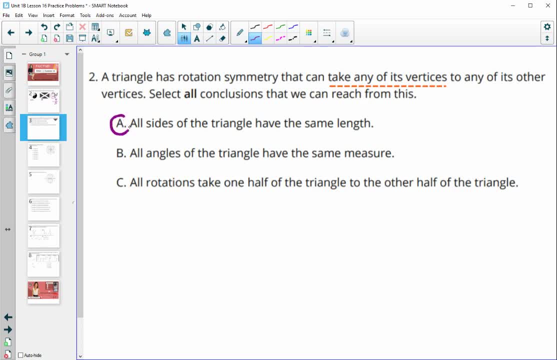 vertex can land on each other. that means that the vertices must be equally spaced for them to land on top of each other and the angles must have the same measure. but it would not count as a rotational symmetry angle. the triangle would end up on the other half. number three: select all angles of. 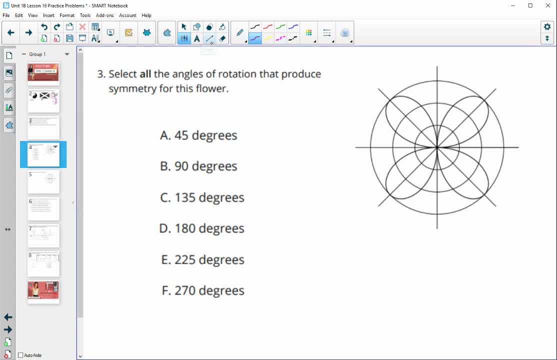 rotation that produce symmetry for this flower. so if we take a look you can kind of see there's four distinct areas here because of these petals. so we would want to rotate this petal around onto this one and then around on to this one, and then around on to this one, and then it would be back. so we'd be looking at. 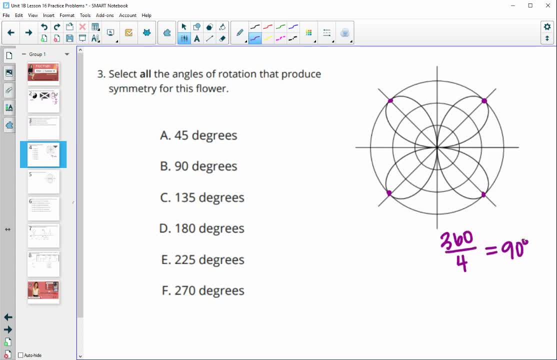 360 divided by four. so every 90 degrees there's going to be rotational symmetry. so not at 45, because then this peak would end up here and that wouldn't be good. so at 90, not at 135, at 180, not at 225 and then at 270.. so this would be the 90, and then 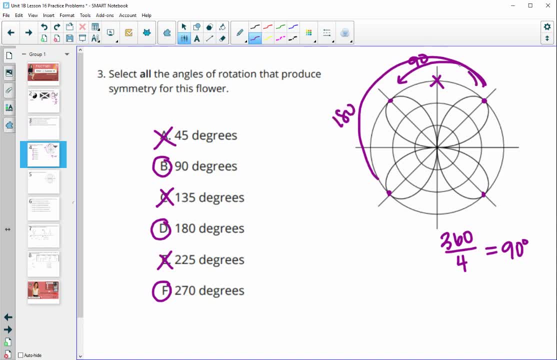 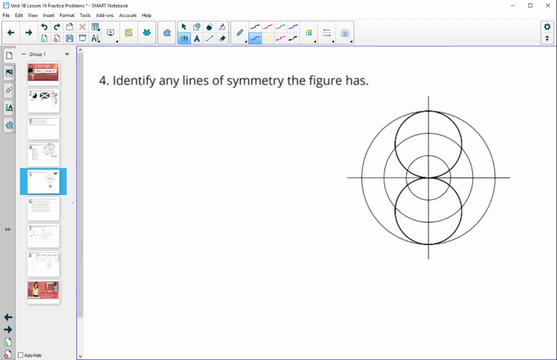 to here would be 180 and then all the way to here would be the 270.. identify any lines of symmetry that this figure has? so we kind of see two distinct parts here, um kind of a top half and bottom half are the same and left and right are the same um. 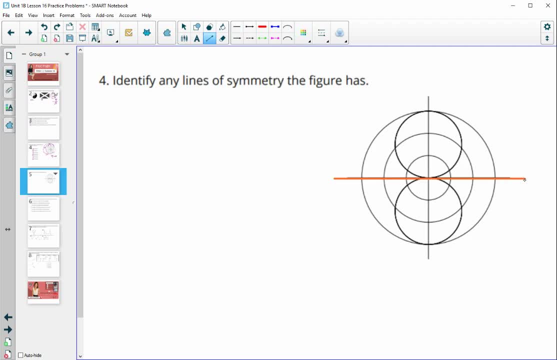 but beyond that really nothing. so this is going to be a line of symmetry that's horizontal and a line of symmetry that's upward and a line is آپ mask up screen. so that's going to be sommes, Це, bZ of symmetry that's vertical, both through the center, so they both have to go through that center. 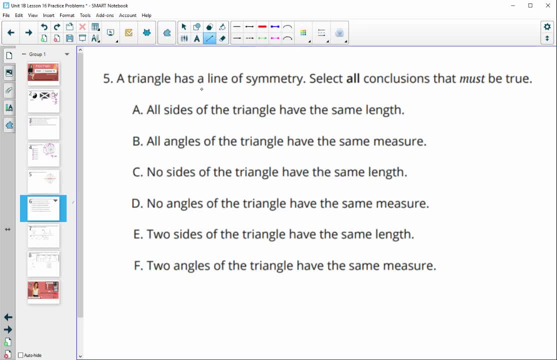 number five: a triangle has a line of symmetry, so one line of symmetry select all conclusions. that must be true. so there is only one line of symmetry here, so all sides of the triangle have the same length. this would not be true, because if that were the case, then this would have symmetry, uh, more than one, because you would. 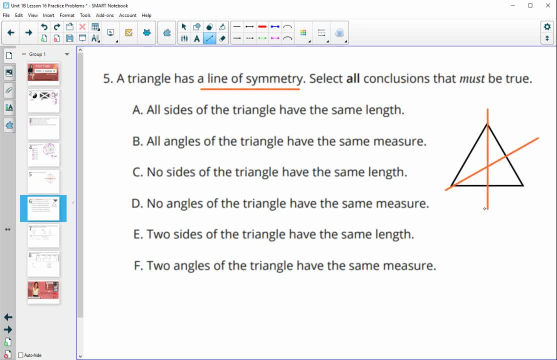 have this one to land on on itself over there. you could fold it this way, and you could fold it this way. so all of the sides cannot be equal, and therefore all of the angles cannot be equal as well, or there would be more symmetry. no sides of the triangle has have the same length. well, 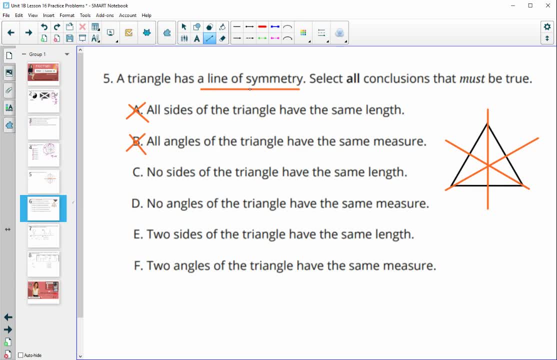 that can't be true if it's going to fold over on itself. by definition, line of symmetry means going to fold over on itself, so it has to have something that's the same. okay, so this would not be true. um, which means same thing about the angles. for the same reason. so two sides of the triangle. 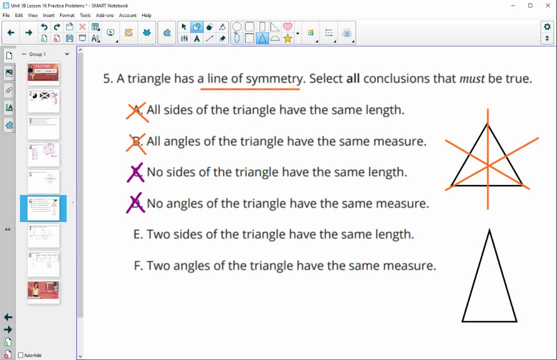 must be the same. so this would be true. so if we had a triangle like this, an isosceles triangle, we would get one line of symmetry there, so then this side would be equal to this side, so it would land it. and then two angles: this angle would have to be equal to this angle so that 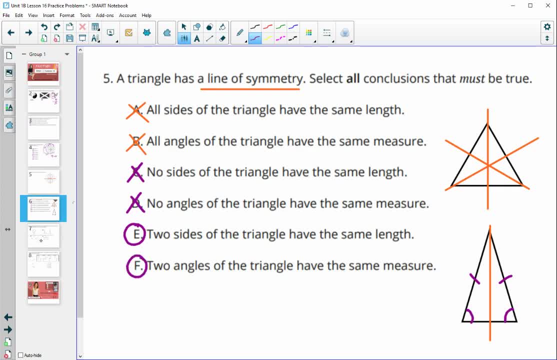 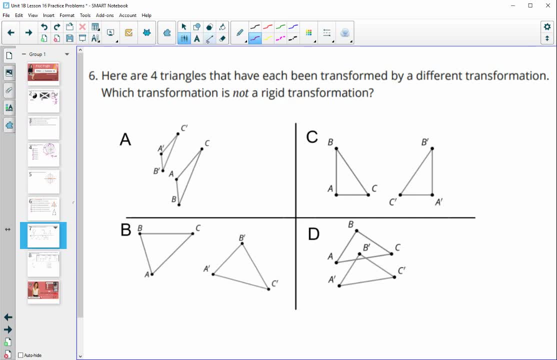 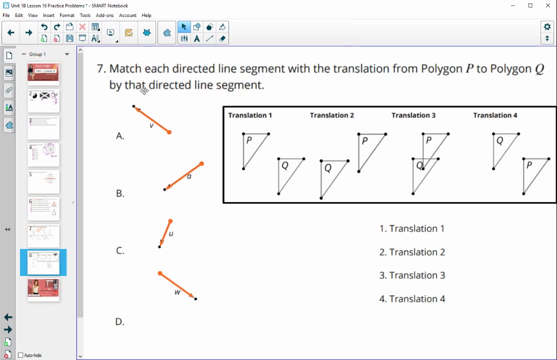 landed on it. number six: here are four triangles that each have been transformed by a different transformation, which one is not a rigid transformation? so remember, rigid transformations stay the same size, so we're looking for a size change, which would be a okay. then, finally, number seven, we're gonna match these vectors to the translations. remember that we are. 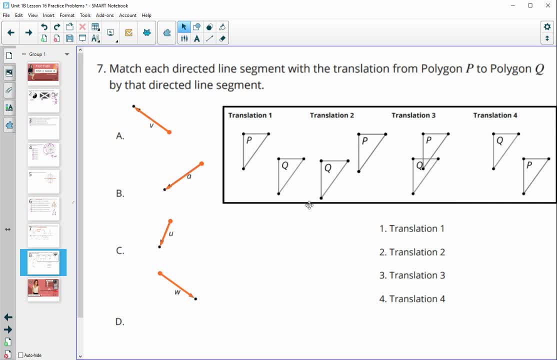 moving triangle P on to triangle Q. so we want to start the vector at P and have the arrow go towards Q. so for this one P should be be be and then up into the left should be Q. So we can match that one to translation number four.